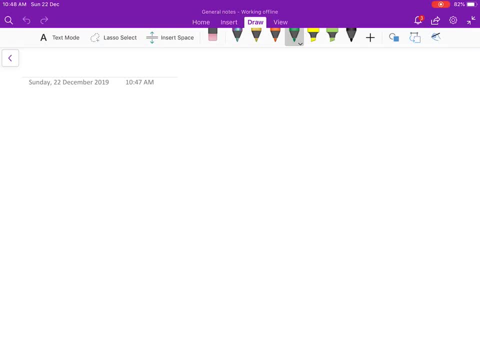 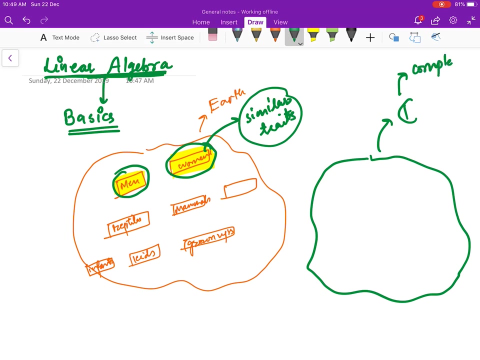 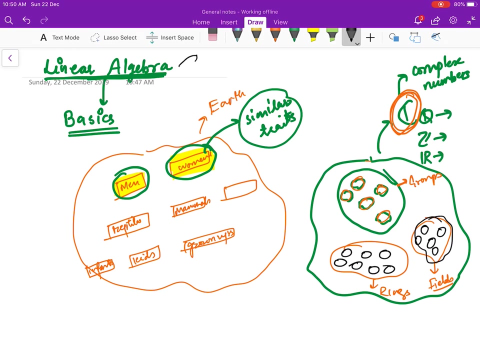 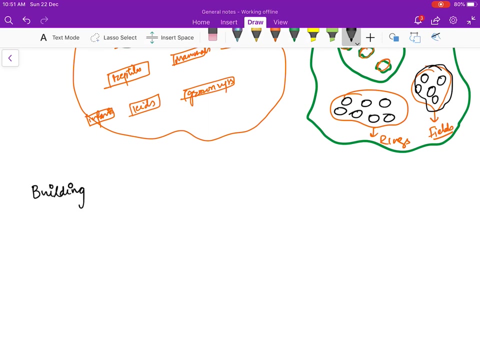 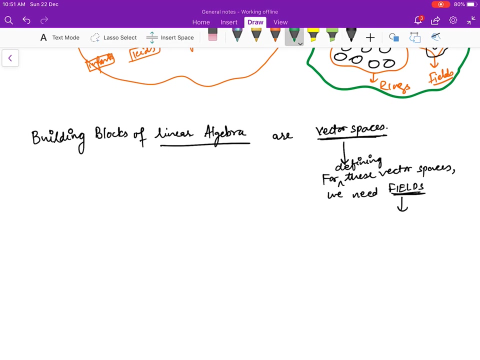 Hello everybody, welcome to this first video on linear algebra. So this is a beautiful subject which we are going to start in this video. And before starting this subject, which like effectively will start in the next video, we need certain you know basics, which we are going to discuss in this video. Okay, so for this basics, I would like to tell you that suppose this is this is the community of everybody who is on this earth. Right? So we know that we love to categorize. For example, we have a category called men, women, or we can have something like, say reptiles, mammals, and so many things, other things. And then we have something. Like kids, infants, and then we have grownups. Why do we categorize? We categorize because a particular community, for example, women, or say men, they have similar traits. You know, so not everything is similar, but they have some kind of similar traits. And, you know, that that is helpful if we are dealing with this particular category of people, or this particular category of people. And similar thing happens in numbers also. Suppose this is the largest set of numbers, say complex numbers. This is complex numbers, set of complex numbers. And inside these complex numbers, we see that they can be grouped, you know, for example, we have Z set of all integers, we have R set of all real numbers, we have Q set of all rational numbers, and so many things, and some smaller groups also. And we would like to talk about this. To, you know, make categories here also, and those categories will be helpful, we will see later on. So the point is, I'm going to tell you, in this set of numbers, and of course, this is extendable, I'm just talking about numbers right now, we have something called groups, we have something called rings, and we have something called fields. These are three, you know, categories of numbers, group sets of numbers, right? So in this category, we have some sets, which follow some similar traits. And similarly, in this category, also, we have some sets, we call these sets as rings. And here also, we have some sets, we call these sets as fields. And these things, generally, these fields, they will be helpful in defining the vector spaces, which are the building blocks of linear algebra. So let me summarize. So building blocks of linear algebra are vector spaces. Let us write it down. Building blocks of linear algebra, which is a subject which we are going to start, are vector spaces, which we do, I assume that we don't know right now. And for defining these vector spaces, for defining these vector spaces, we need fields. And this is what we are going to define in this video. And before fields also, I will define something called binary operation. 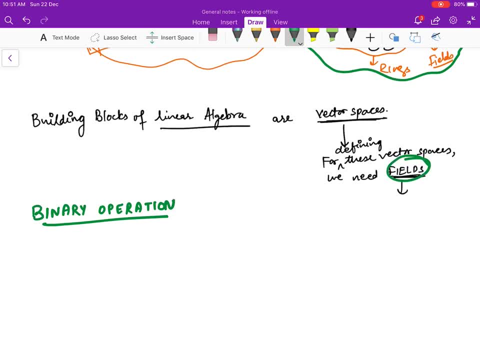 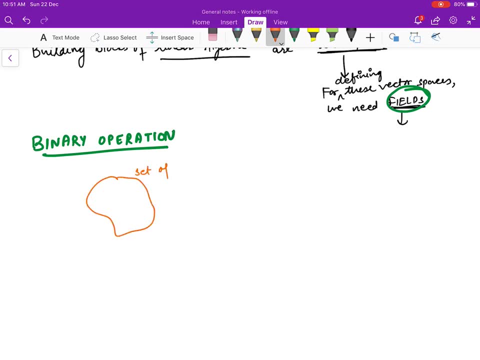 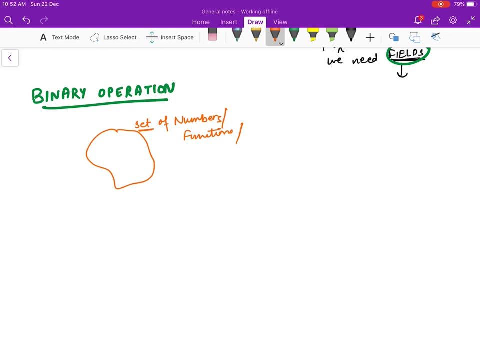 So we are in this direction of defining this field. So this starts from here. So something called binary operation. So what is the binary operation? Suppose you have a set, set of numbers, or it can be set of functions also, set of polynumbers. It can be anything. So right now, you have a set, which can be set of numbers, functions, or any mathematical entity. Okay, so we say that you have, you have an operation, you call this set as a. So you what you do, you make a copy of this set a, right, and you pick one element from here and one element from here. And you do something with these two elements. And that's something say cross. So you have a here. and say b from here and you are crossing a and b and if this a cross b again belongs to a again belongs to a to the set a then we say that this cross is a binary operation 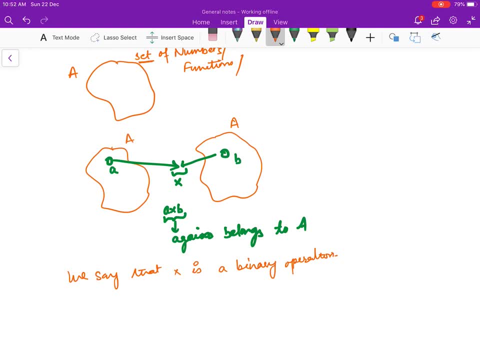 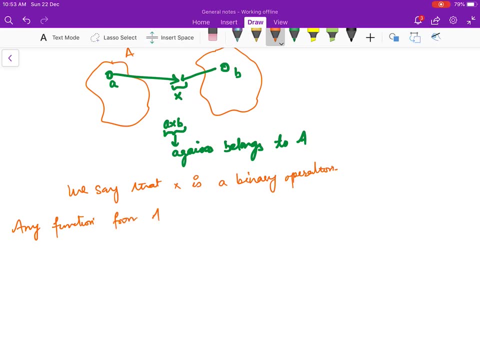 right so the definition is mathematical definition is any function from a cross a to a is a binary 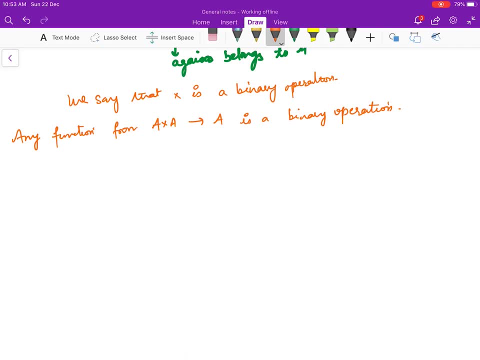 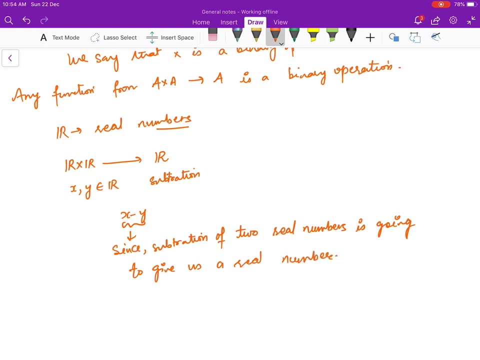 operation so let us see the examples so you can have say you have a set of real numbers right set of real numbers and you you define from r cross r to r an operation where you take x and y from r and then you define the subtraction. So, you have x minus y. Now, you know that if you subtract two real numbers, you are going to get for sure a real number. Since subtraction of two real numbers, two real numbers is going to give us a real number. So, we know that this subtraction 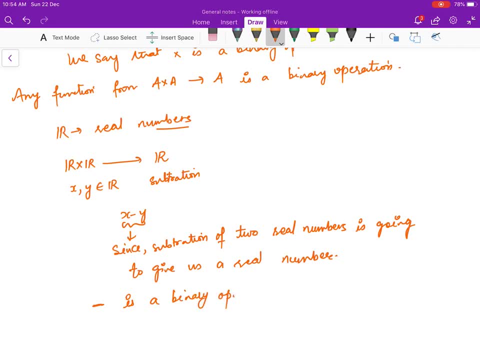 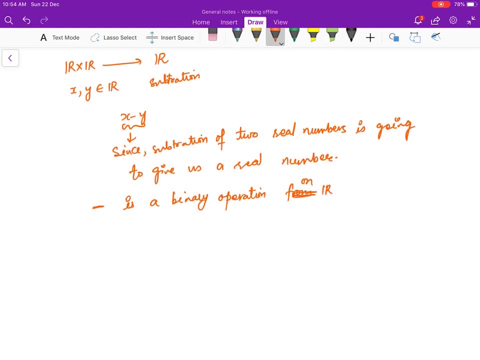 is a binary operation from r on r. Okay. Now, let us see this is not a binary operation. So, you can. 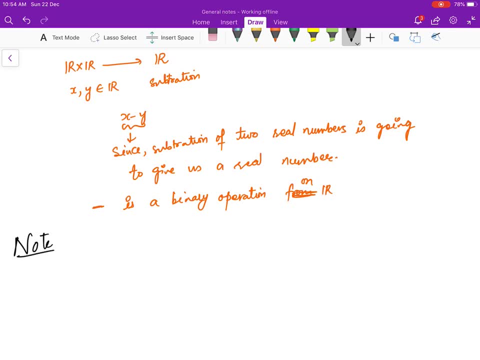 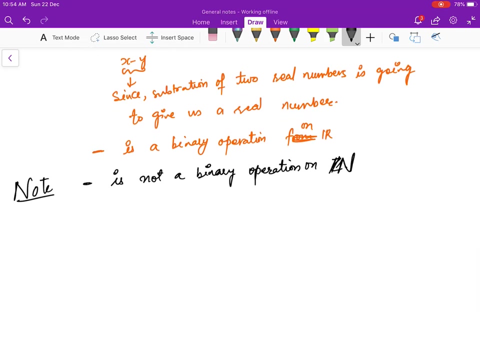 Note this thing. Subtraction is not a binary operation on z. How? Not on z, on n, set of natural numbers. Right. So, because we know that if you take two natural numbers, say 4 and 5 and you subtract these two natural numbers, you will get minus 1 which is not a natural. 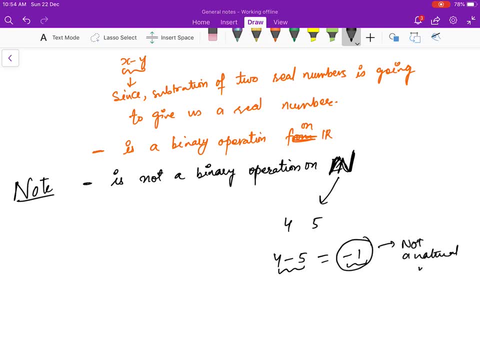 cherry is h is not a natural number. So, subtraction is not a binary operation on set of natural numbers. Okay. So, this was what is a binary operation. Now, let us define what is a field. 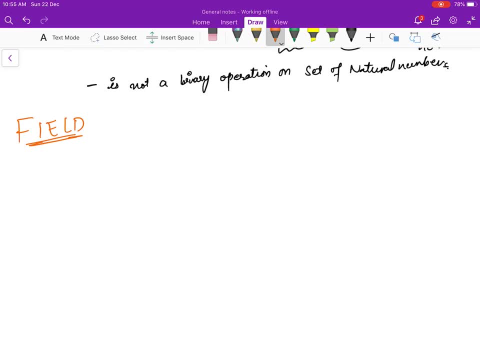 Before that, actually, we should go from group to ring and then field, but because we are going to this you know I want to be specific whatever is required in linear algebra so that is why I am not going into those things that what is the group and we can have that thing separately so what is the field field is a set f you have a set f then you have two binary operations this can be anything this is just a notation I denote these two binary operations with addition and multiplication so these are two binary operations so a field is always a set with two binary operations satisfying certain properties so let us look at what are those properties so the first properties of course I have already called 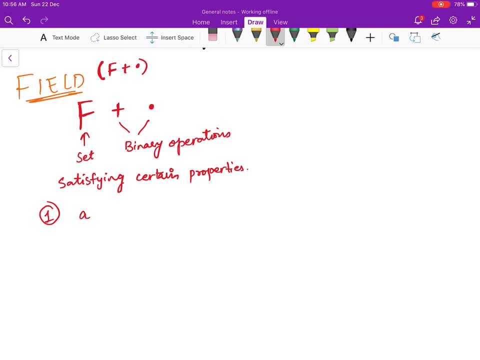 these as binary operations. But let me write it down. Let me write it down that if I take any two elements from the set f then these two operations will lead to the same element from the same set for all a b belongs to f this is nothing but this is same as saying plus and dot are binary operations this is what we have already 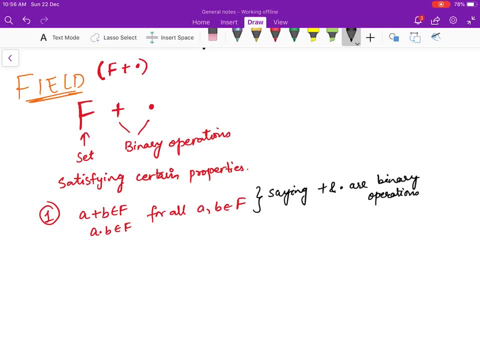 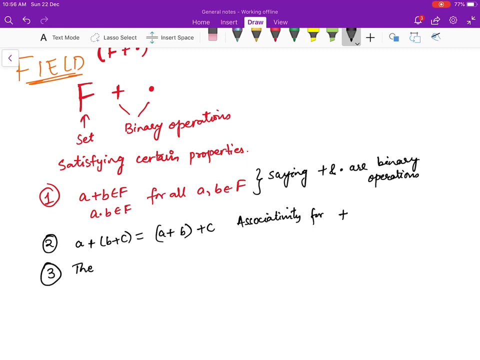 said right so this is the first thing which is required then the second thing is that you have to come up with the associativity for the plus a plus b plus c should be same as a plus b plus c so this is called associativity for addition then you have identity for addition there must exist an element. 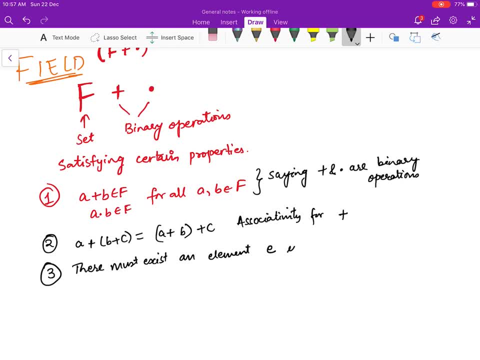 Say E in f such that a plus e is greater than f. Let me write this down. Let me write this down. So this is the first one. 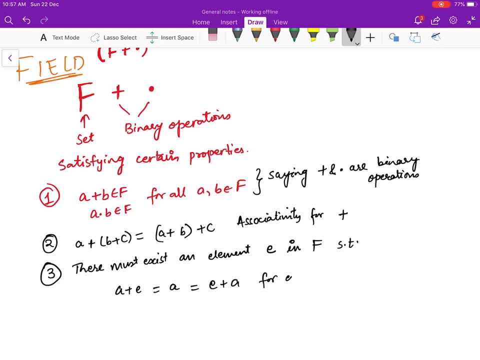 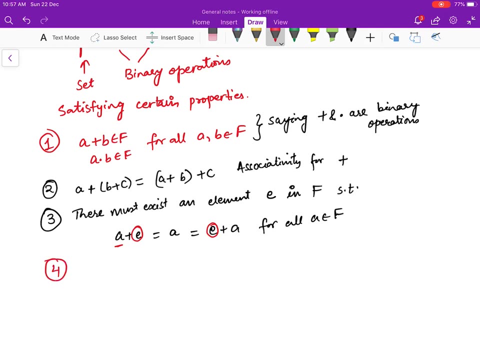 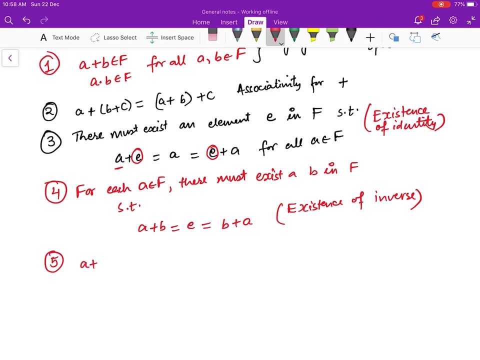 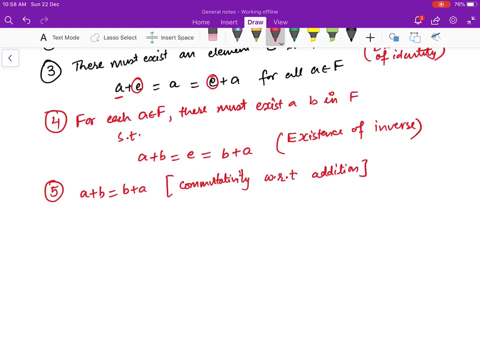 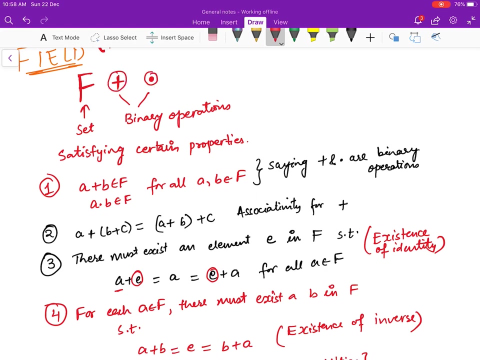 should be equal to a equal to e plus a for all a in f means that there must be an element in your set you know which will not affect the element if we add that element to all the elements of f the fourth property is this is called existence of identity then fourth properties for each a in F there must exist a B in F such that a plus B is equal to e is equal to B plus a so this is called existence of inverse and then the fifth property is a plus B should be same as B plus a this is called commutativity with respect to addition right then the sixth property is you know now we are done with addition we have to come to this multiplication and I want to make a point that this is not the addition it can be any operation we are just calling it as an addition 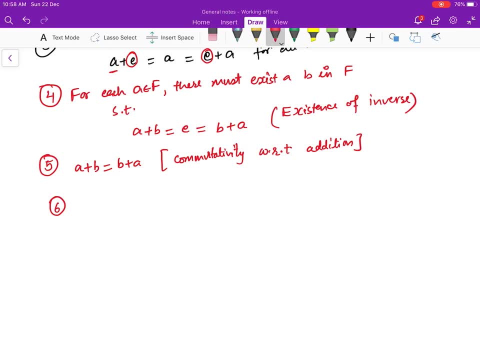 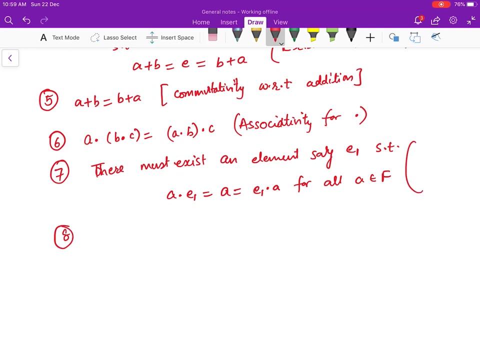 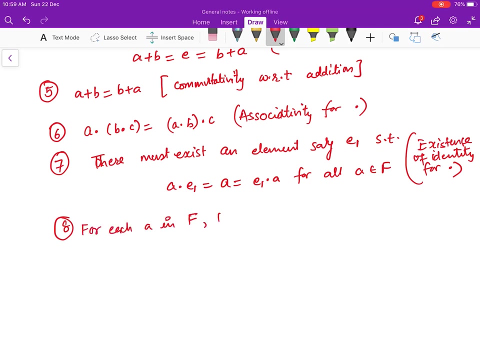 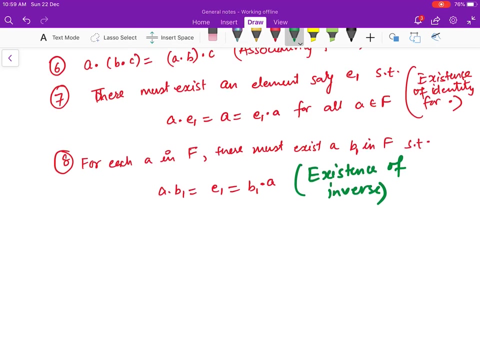 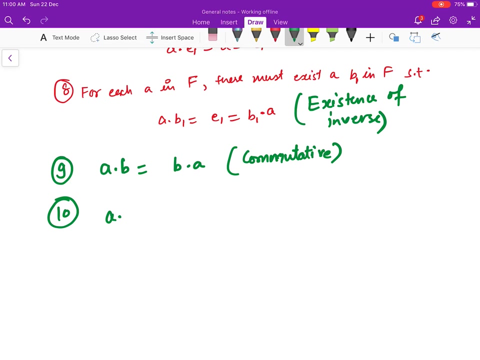 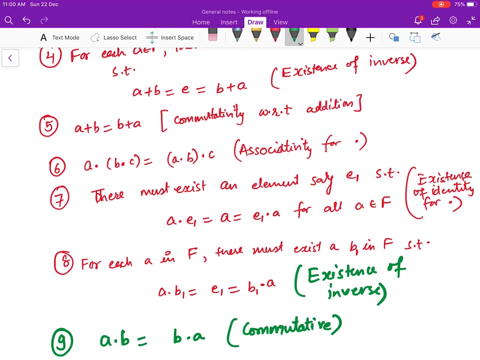 so the properties for multiplication they are associativity again a dot B dot C should be same as a dot B dot C so this is associativity for dot then you should have identity for that so there must exist there must exist an element and say now let let us call it as E1 such that a dot E1 is equal to a is equal to E1 dot a for all a in F and then this is called identity existence of identity for dot existence of identity for dot then the next is for each a in F there must exist a b in f it will be b1 say such that a dot b1 is equal to e1 is equal to b1 dot a for all this we have already written for all a okay this is called existence of inverse for multiplication of course and then we have commutativity for multiplication that is a dot b is equal to b dot a this is called commutativity the last one is a property combining these two operations so we should have dot should be distributive over addition so a dot b plus c should be a dot b plus a dot c and a plus b dot c should be a dot b plus a dot c and a plus b dot c should be a dot b plus a dot c and a plus b dot c should be a dot b plus a dot c plus b dot c so these are the 10 properties you see if these 10 properties 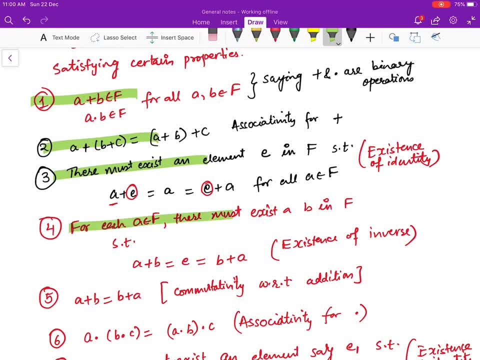 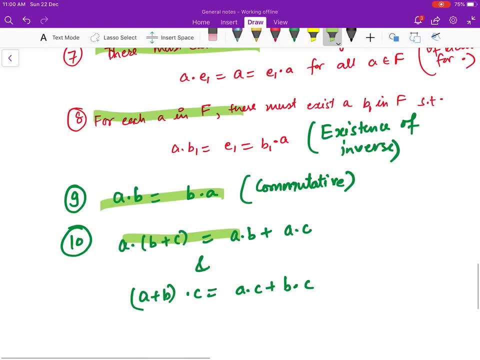 are satisfied this is the first one second one third one fourth one fifth one sixth seventh eighth ninth tenth and these 10 properties are satisfied we say that this set together with these 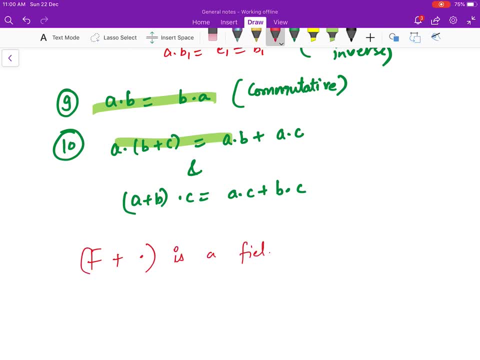 two operations is a field right so whatever we required in the vector spaces definition is we should know that this r 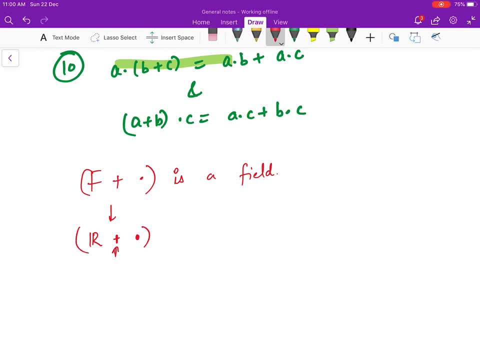 r over this normal addition which we know and this normal multiplication is a field and c complex numbers with addition and multiplication is a field so uh is a field let us see how this r let us see r plus dot so we know that first of all these two should be